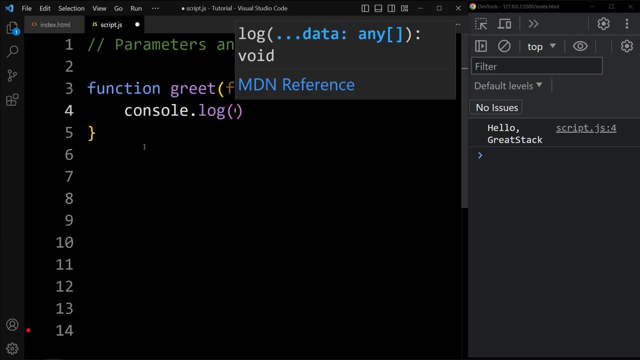 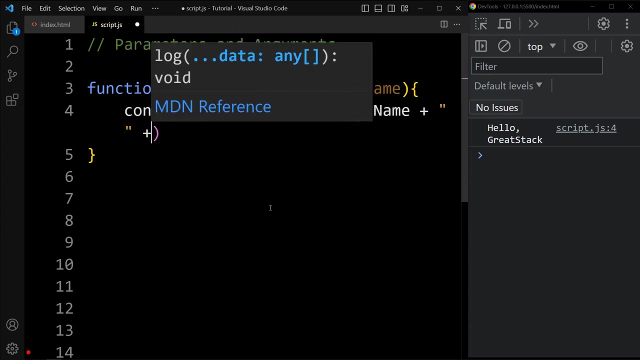 add console dot log And we will add the text Hello, plus. there will be first name, Then we will add plus and one space within double quote. Then again we will add plus and last name. So it will print hello, first name and last name in the console tab. So right now we have declared the function with 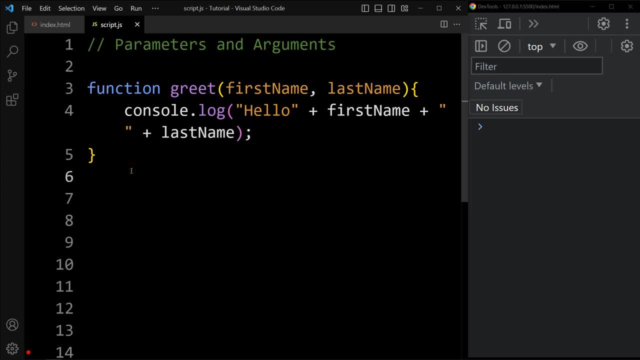 two parameters. Now we have to call this function. While calling this function we have to pass two values that will be arguments. So to call this function we will add the function name greet, And with this function name we have to add two values. So let's add first value, Elon comma. 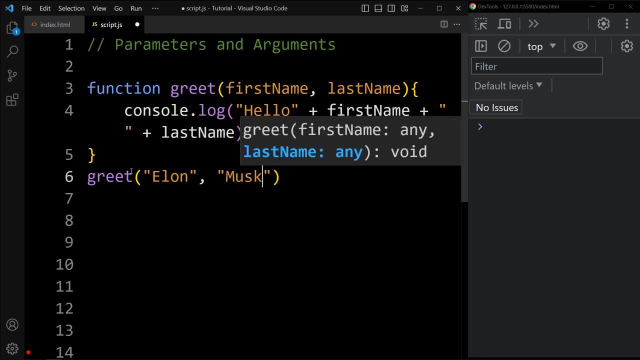 greet And this function name. we have to add two values. So let's add first value: Elon comma Musk. So we are passing two values when calling this greet function. Now you can see the output in the console tab Here it is printing: hello Elon Musk. Let's add a space here. 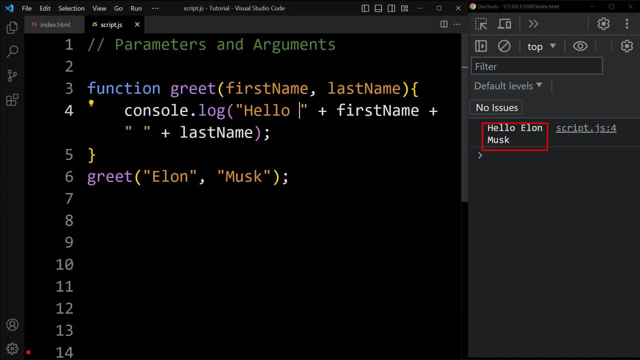 Now it looks good. Hello, Elon Musk is printed in this console tab. We can pass any data type as argument. So let's add another data type as a function. Here I will add 200.. That will be number. Here also we will add 100.. Now see the. 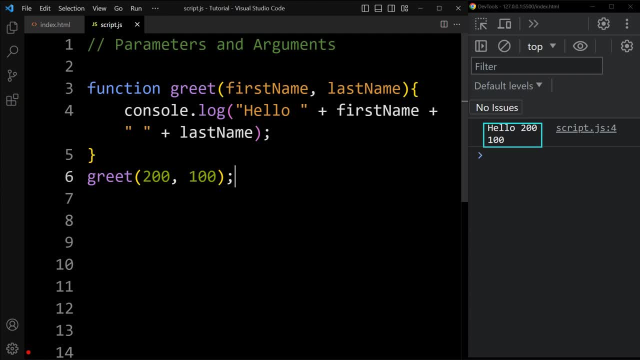 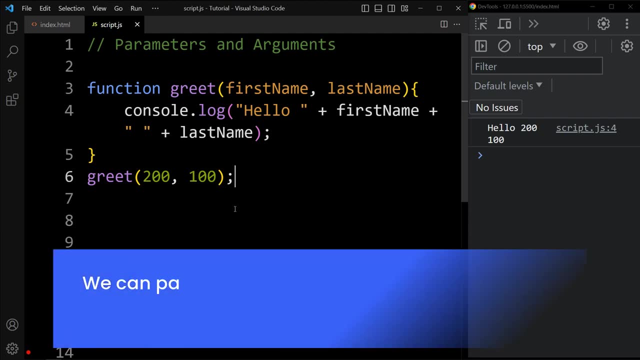 output. You can see it is printing hello 200 and 100. So we can pass any data type as argument while calling the function. We can pass less or more arguments while calling a function. If we pass less arguments, then the rest of the parameters will be undefined. If you pass more arguments, then 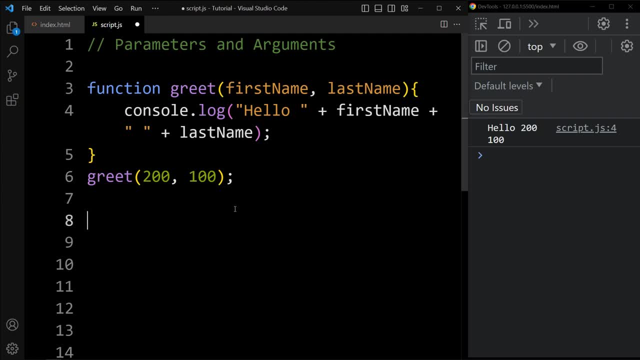 arguments will be ignored. Let's see one example. If I just pass greet Elon and comment this first call, Here you can see the output. It is saying: hello Elon. and undefined, Because we are passing only one argument and here we have two parameters, first name and last name. So this Elon 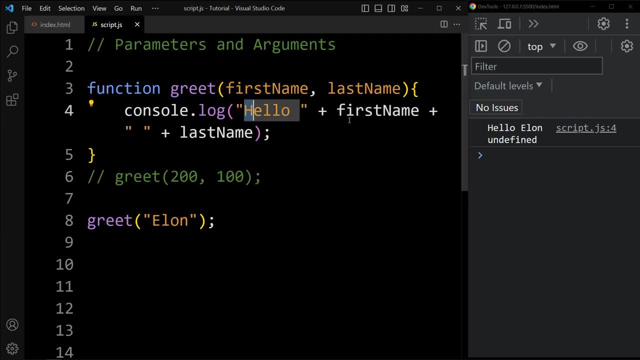 is stored in this first name, So it will print hello and the first name is Elon. And in the second parameter, which is last name, we are not passing any argument, So it will be undefined. That's why it is printing hello, Elon, undefined. The last name is undefined, So we can pass less argument. 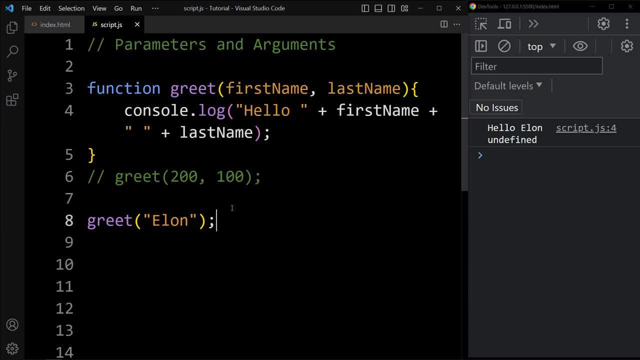 Now let's see another example. if you pass more arguments Here, if I add Elon, comma Musk, Comma Mr. Now see the output Here. it is printing: hello Elon Musk. So the first argument will be stored in the first parameter, which is first name. 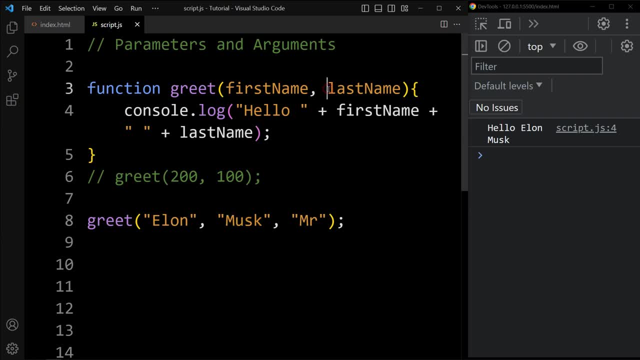 Second argument will be stored in the second parameter, which is last name, And this third parameter will be ignored, Because we have only two parameters here, So it will only print this hello And the first name will be undefined And the last name will be undefined And the first 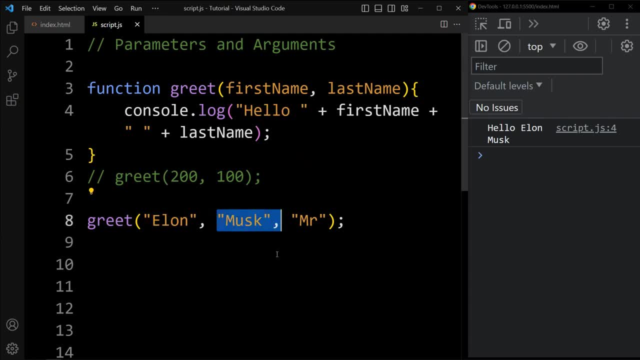 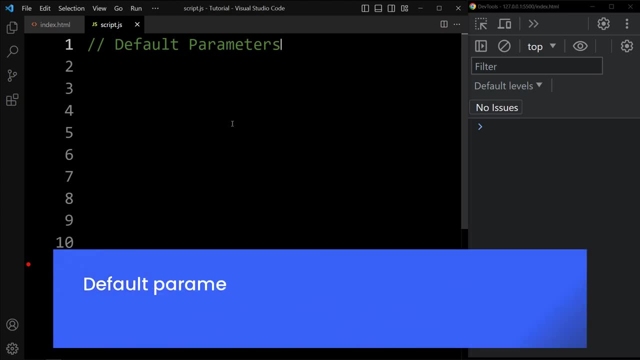 name Elon and last name Musk. The third argument will be ignored. Now let's learn about default parameters. Default parameters in JavaScript are parameters that have a default value. This means that if the argument is not passed to the function, the default value will be used. Let's see one. 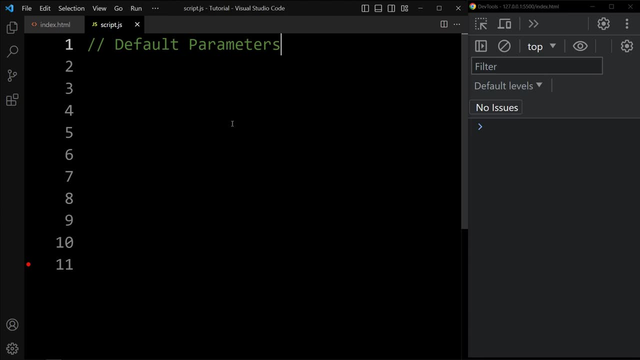 example of default parameters. Here we will create one function, Write the function name, Sum, And in this sum function we will add two parameters, which is x and y. Now in this body of function we will add console dot log and it will log the x plus y. It will add: 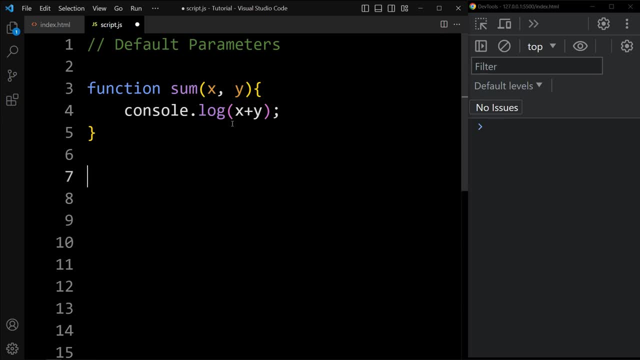 the x and y value and it will display in the console tab. Now to call this function, we will add function name and parenthesis. But here you can see we have two parameters, x and y. So when calling this function we have to pass two arguments also. So let's add two values: 10 comma 15.. So this 10 will be stored in x. 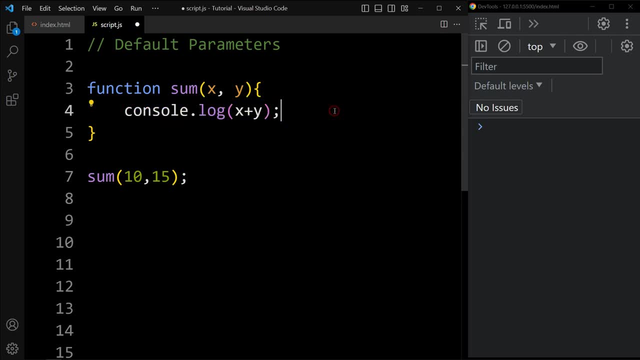 15 will be stored in y And this console dot log will display 10 plus 15.. That will be 25.. You can see in the console tab it is printing 25.. 10 plus 15.. Now you can see if I remove 15 from here and we are just passing 10.. 10 will be stored in x and y. 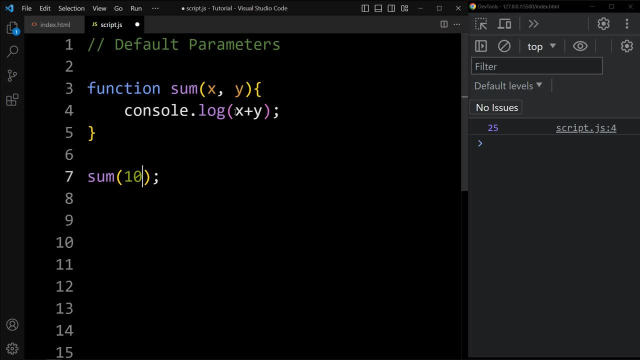 will be undefined, And here we are printing x plus y. So let's see what will be output. Here it is printing nn. Why? It is because here we are adding 10 plus undefined. x plus y will be 10 plus undefined. 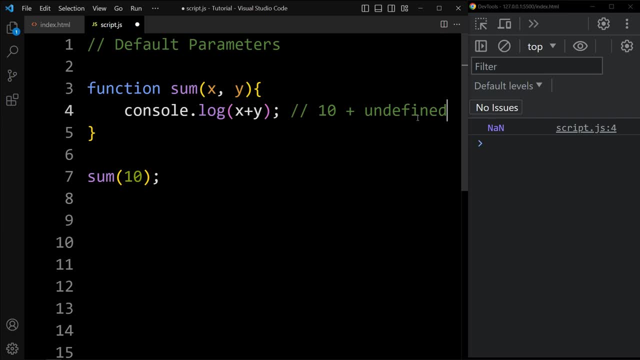 that's why it is printing nan. that means not a number. we cannot add the undefined n number, so it is printing nan. here we are passing only one parameter and you want this function to work. for that we can add: y is equal to 0.. suppose we have added y value 0, then you can see the output. 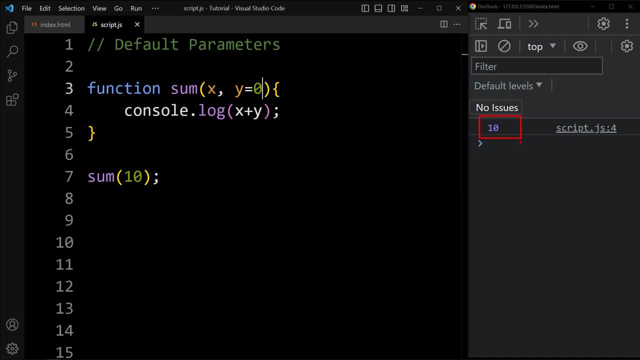 in the console tab. it is printing 10.. let's see if i add 50, we are passing 50 in x and y. default value is 0. so x plus y, that means 50 plus 0, that will be 50. you can see the output. 50 is printed. 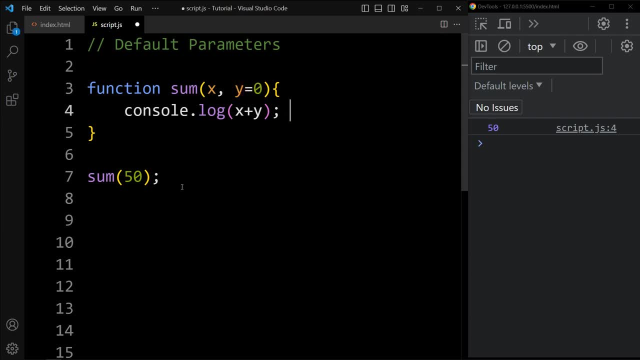 so 0 is the default value of this y parameter, and here if we pass two numbers, 50 plus 30- then it will use 30 in this y you can see the output: 50 plus 30. 80 is printed here because we are passing two arguments: 50. 50 will be stored in x. 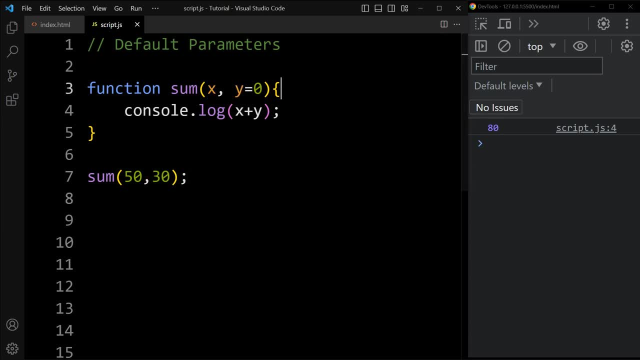 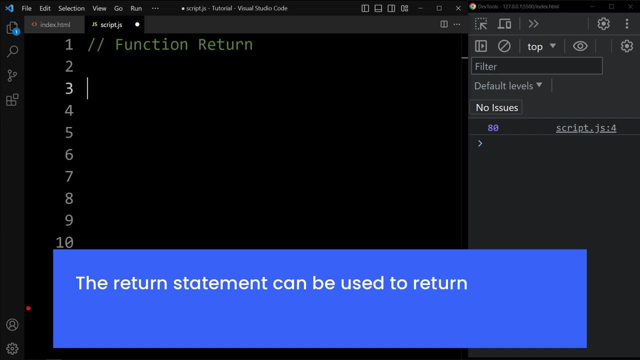 30 will be stored in y, so this was the default parameters in javascript. now we will learn about function return. the return statement can be used to return the value when the function is called the return statement. and when the function is called the return statement, it means that the function has ended. 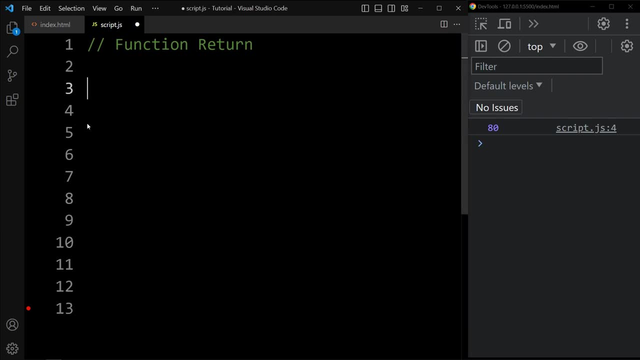 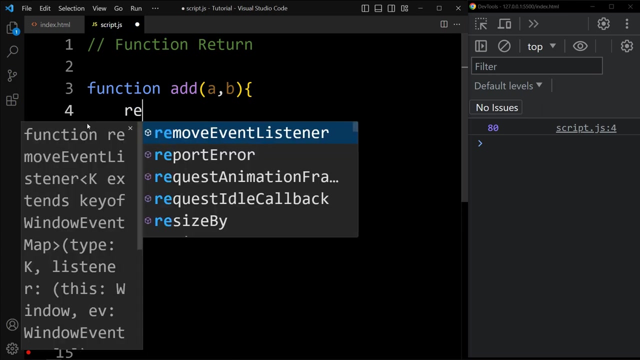 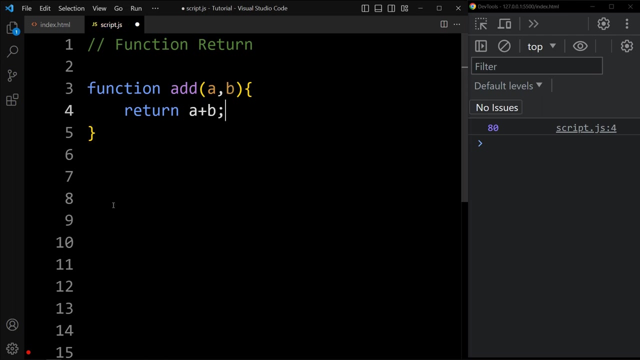 any code after return is not executed. let's see one example. if i create one function and function name is add, and in this one we will add two parameters, a and b, now we can add return a plus, So this function will return the addition of a and b. 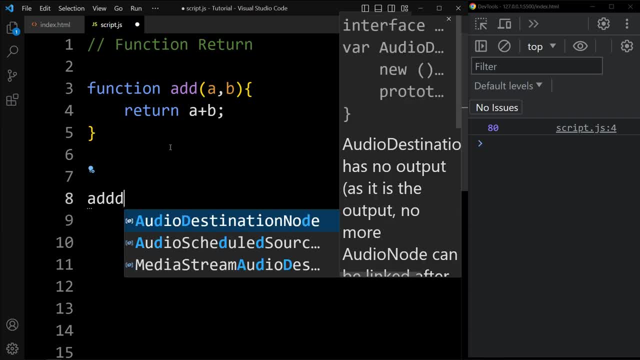 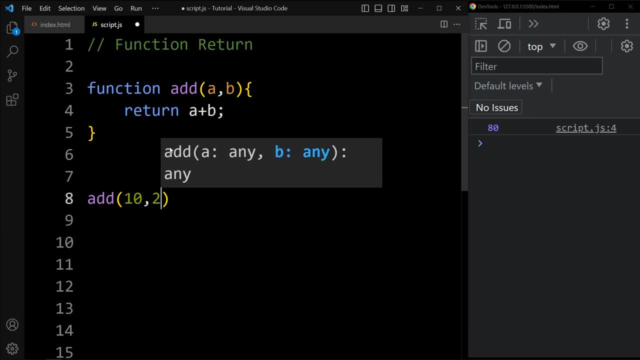 Now to call this function, we will add the function name add, and in this one we have to add two values as argument. so we will add 10 and 20, so this will call this function and this function will return the addition of 10 plus 20, so we can store this result. 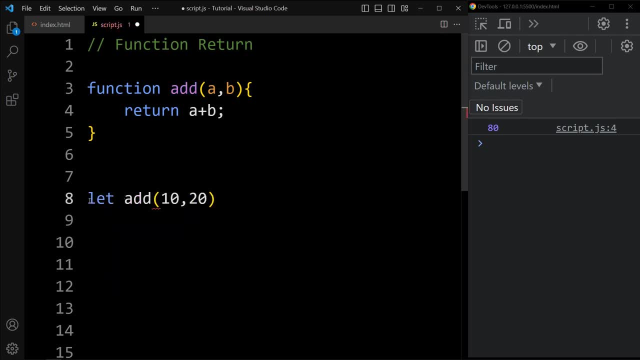 so here let's add one variable with the let keyword. let result equal to add function. so the return of this add function will be assigned in this result variable. Now we can print this result. we will add console dot log. The sum is 20.. 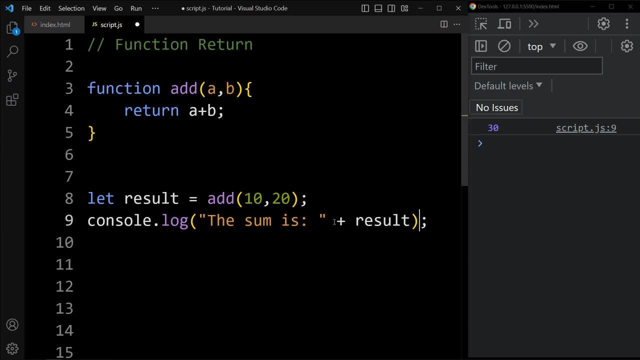 Okay Result. Now you can see the output in the console tab. it is displaying the sum is 30.. If we add 10 and 40, you can see the output in console tab- the sum is 50.. So this return statement will return the value. 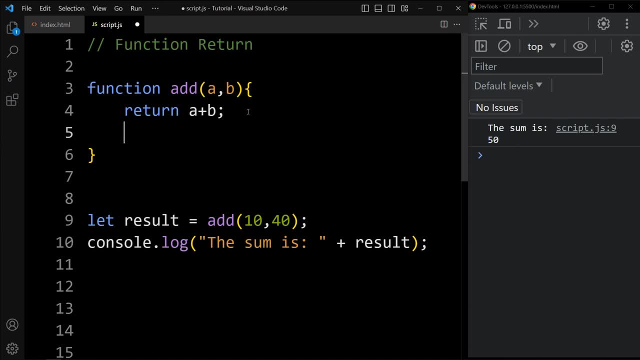 If we add any code after this return statement, like a multiply by b, this code will not be executed. Return statement denotes that the function has ended. Any code after this return statement will not be executed. In JavaScript, a function can return another function also. 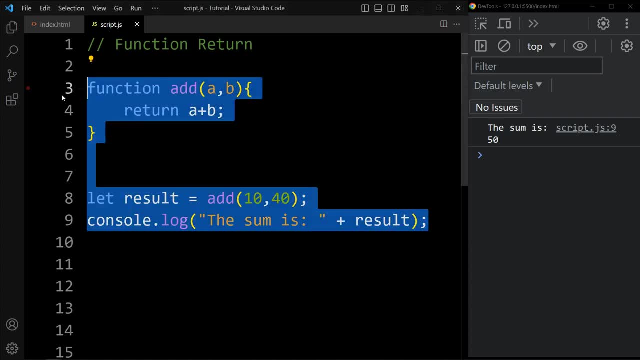 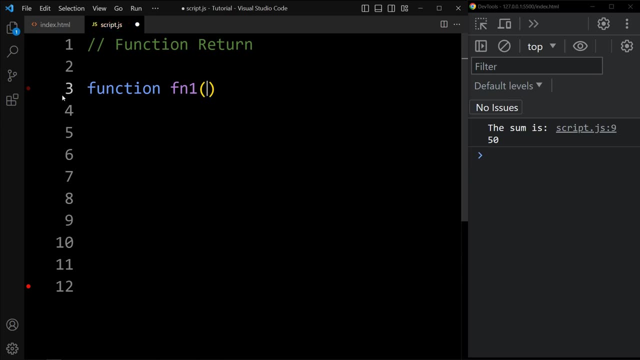 Let's see one example Here. if we create one function with the function name fn1,- so this is the first function Here I am adding one parameter x In this function 1, we will create another function. Let's create function fn2, and this will accept one parameter y. 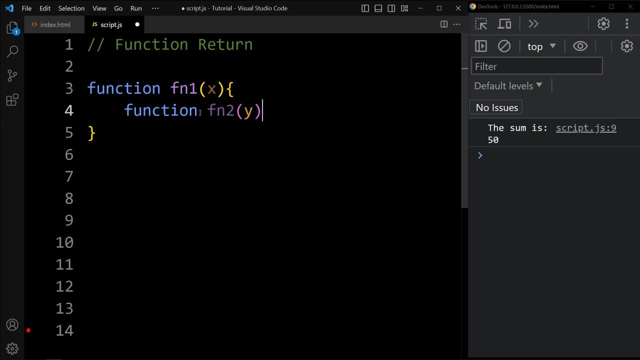 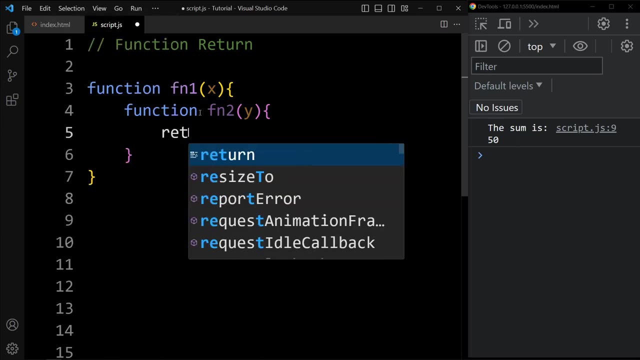 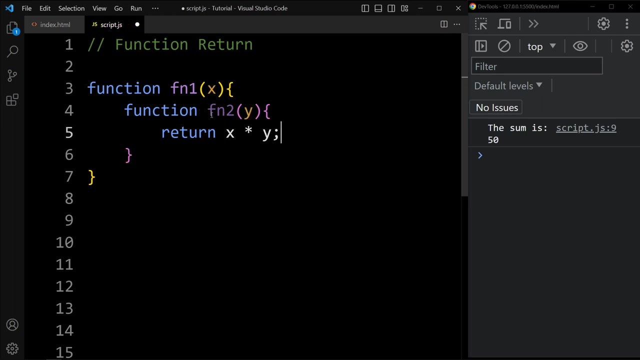 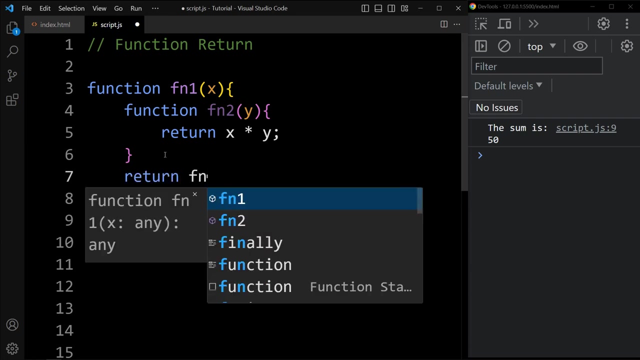 Now in this second function, we will add return x multiply y, So the function tool will return the multiplication of x and y. Next we will add the same thing. Next, after this function 2, we will add return fn2.. 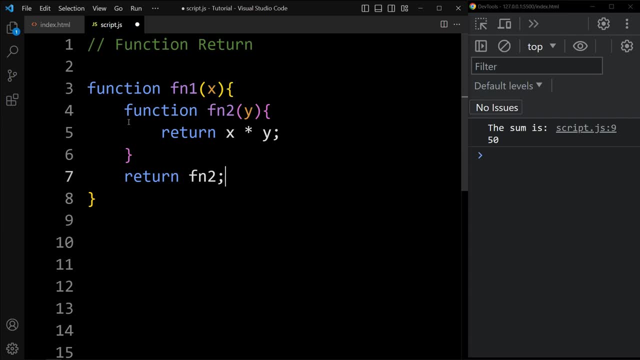 So when we will call this function 1, it will execute this function 2 also and then it will return this function 2.. So function 1 is returning another function, that is function 2. So to call this function, we will add fn1 parenthesis and we will pass one argument. 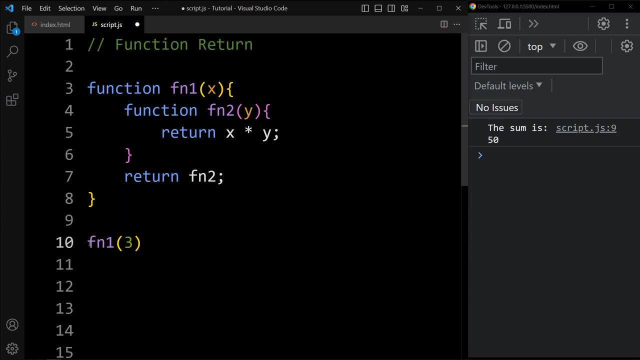 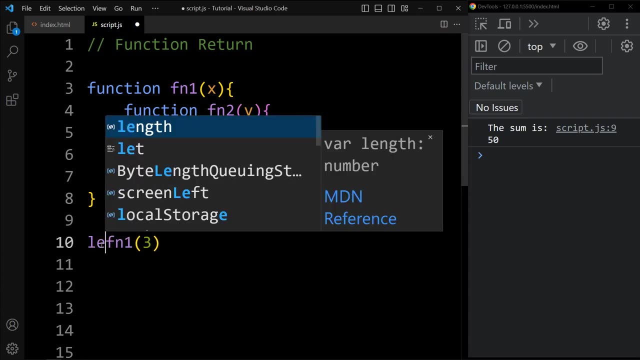 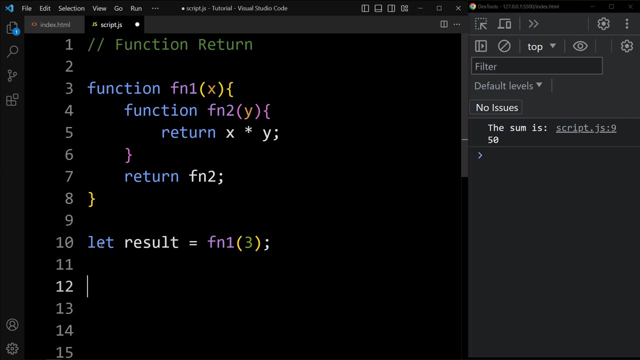 So let's add 3.. So here we are calling function 1 and passing one argument. Let's store its value in one variable. We will add let. result is equal to function 1 and try to print this result: Console dot log. 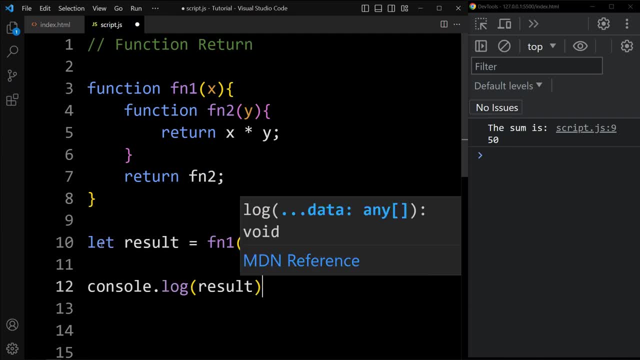 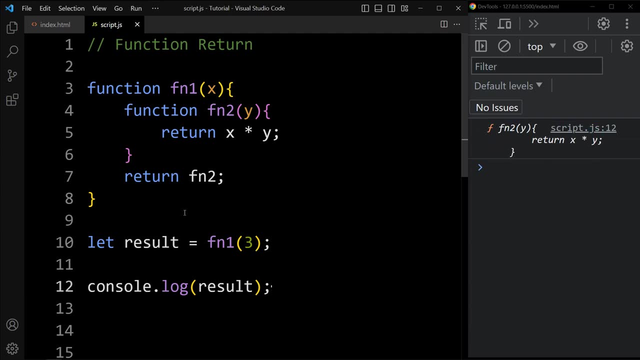 Result. So you can see the output in the console tab. Here it is displaying one function, So you can see when I am calling this function 1, it is returning the function 2 and that function 2 is stored in this result. 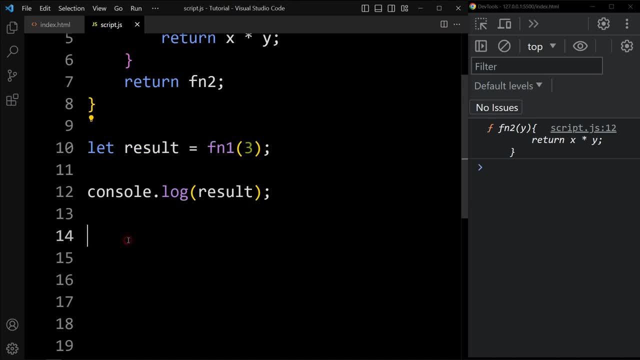 Now the function 2 is stored in this result, So we can simply call this result like this Result For the second function. also, we need one argument, So we will add 2.. And let's print this one. 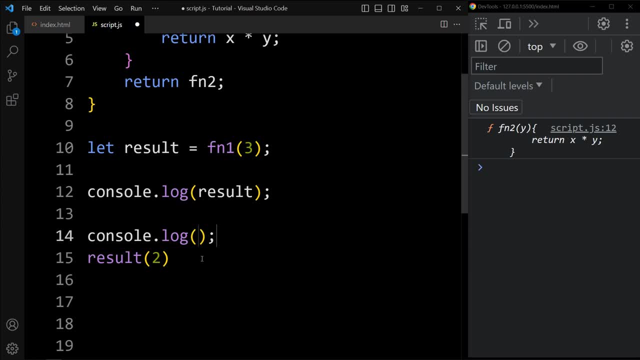 We will add console dot log and print this result to. you can see the output. It is displaying 6 because in function 1 I am passing 3, that will be x, and function 2 I am passing 2, that will be y, and x multiplied by y will be 3, multiplied by 2 is equal to 6..